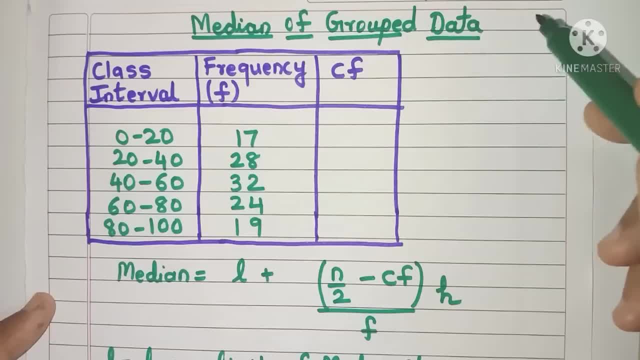 Hello everyone. today we will be finding the median of group data. Now this is the class interval column and this is the column with the frequency values. Now the median formula is given by L plus n, by 2 minus cf, divided by f into h. So before we use this formula, friends, we need to. 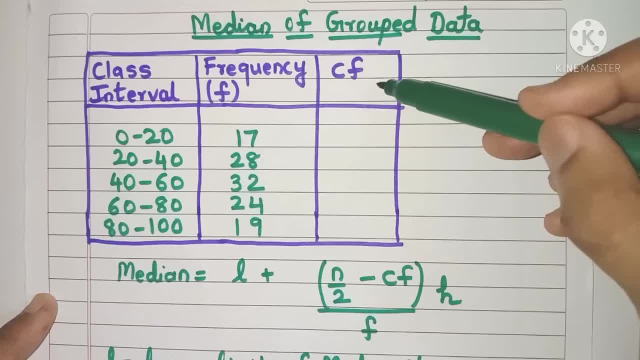 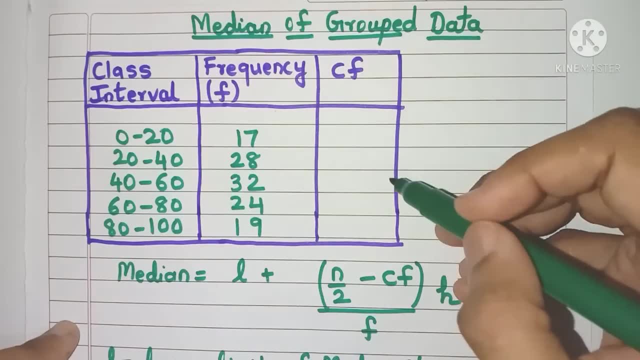 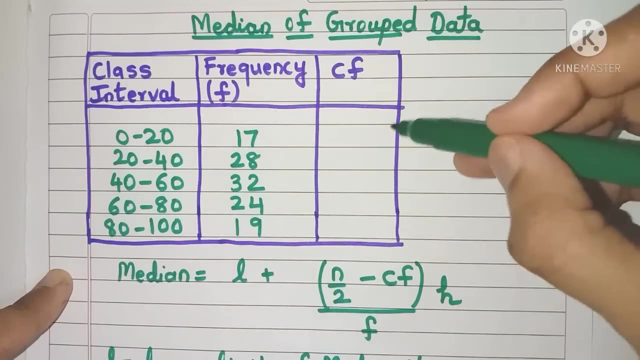 write a new column called the cf, that is, the cumulative frequency column. So what is cumulative frequency? It is nothing but the added frequency. So how to write the values? So for the first class interval, the f value and the cf value are going to be the same, because there is no previous. 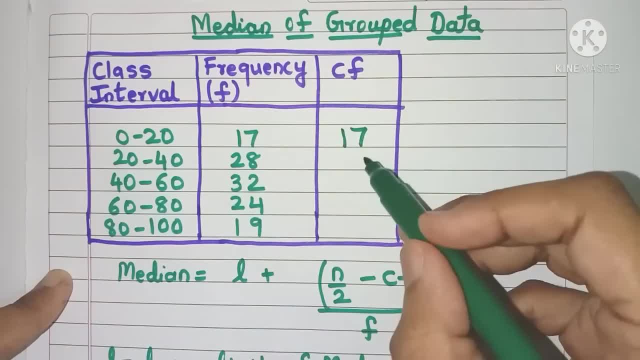 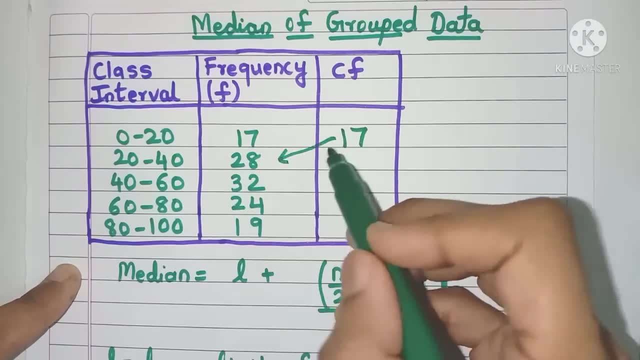 frequency, So we'll write 17 only over here. Now for the next class interval, you simply add the previous cf with this frequency, So 17 plus 28.. How much will you get? 45.. Okay, this is the cf. 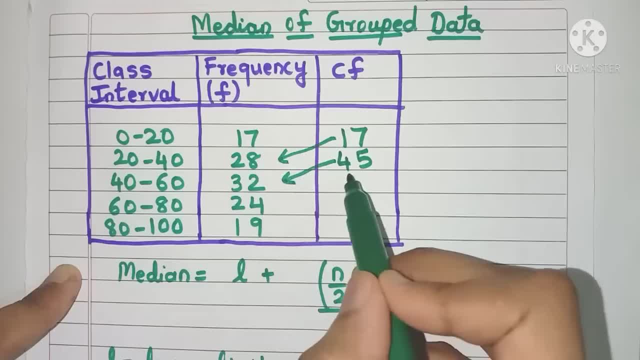 value In the same way: 45 plus 32.. What will you get? 45 plus 32.. So this is the cf value. So you get 77.. That will be the cf. Now, again for this cf, you take the previous cf, add it to 24.. 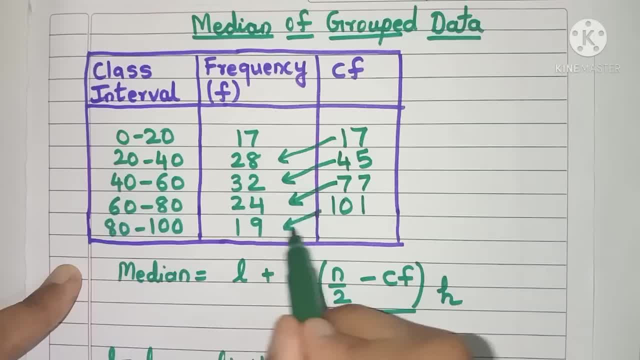 You will get 101.. Then again, 101 plus 19.. What will you get? 120.. So this is how you have to fill out the cf column Now. at the end, you will get the total as 120.. Now, this 120 is nothing but. 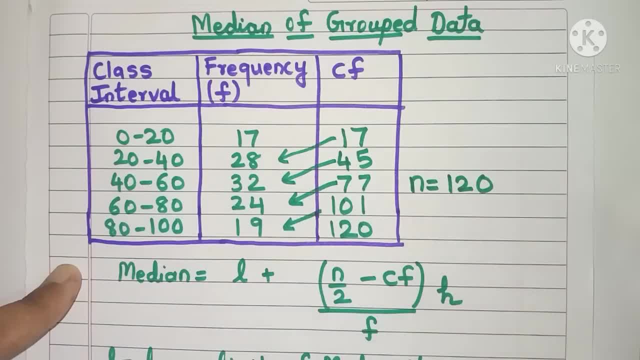 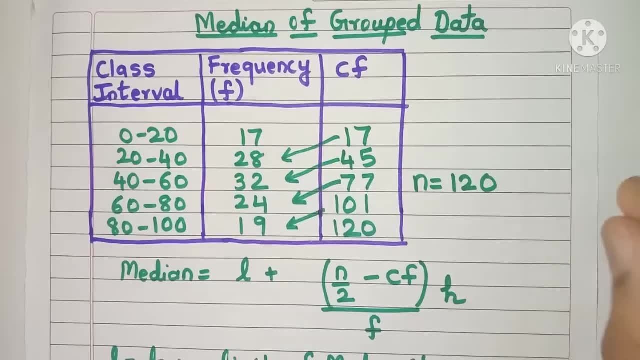 the total number of observations. So, even if they don't give in the question: how many observations are there? you can easily find this out using the cf. So, friends, now we need to find: where does the median value lie? What is the position? So for? 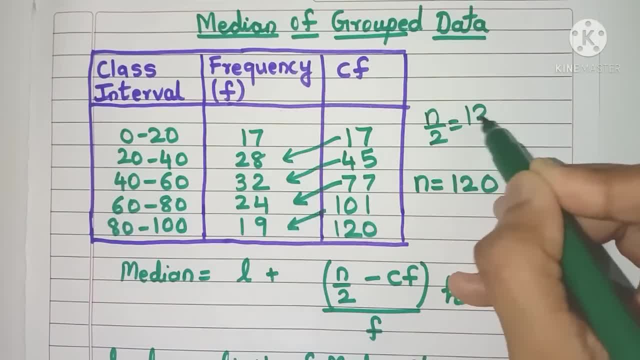 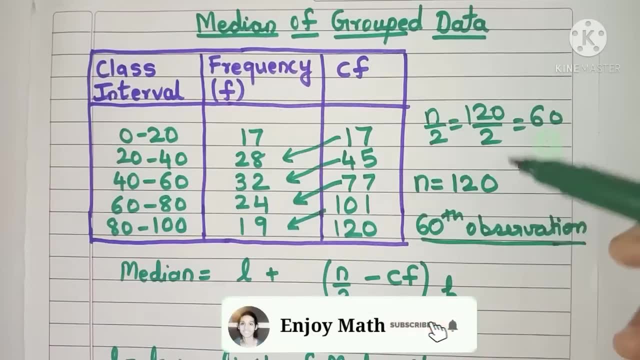 that we need to divide n by 2.. Okay, that is 120 by 2, we'll get 60, which means the median lies on the 60th observation. Now, how do we know? where does the 60th observation lie? In which class? 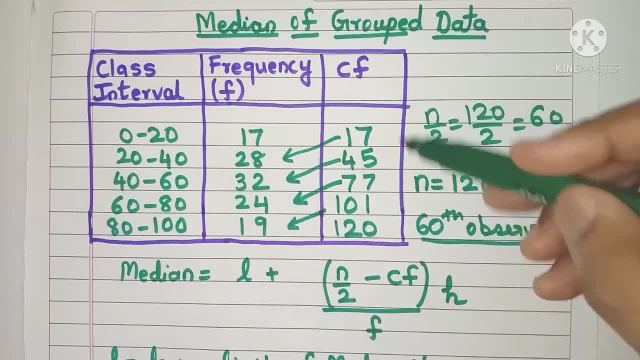 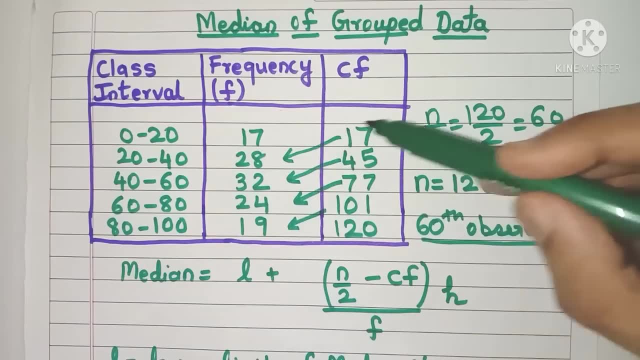 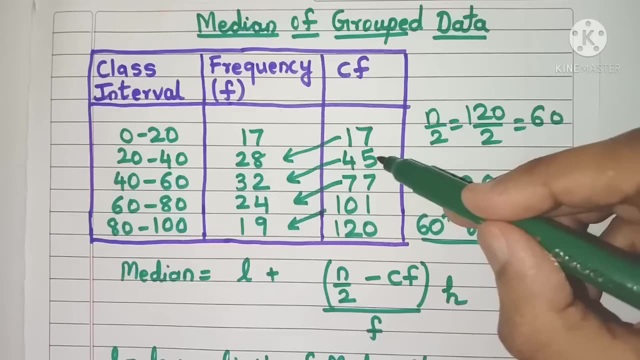 interval. does it lie Now? for that again we need to make use of the cf column. So let's start from here. That means observation number 1 to 17 lie in this class. So 60th observation obviously will not lie Here. also it is observation number 18 to 45 is lying in this class. Again, 60 will not be. 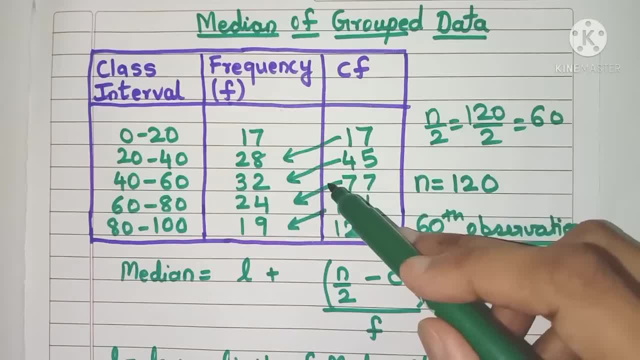 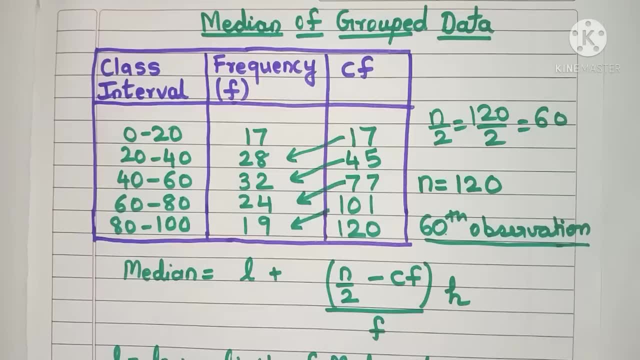 here Now in this class you have observation number 46 to 77. That means my 60th observation will definitely lie in this class. That means this is my median class friends. So I hope you understood this: how to find the median value. So let's start from here. So let's start from here. 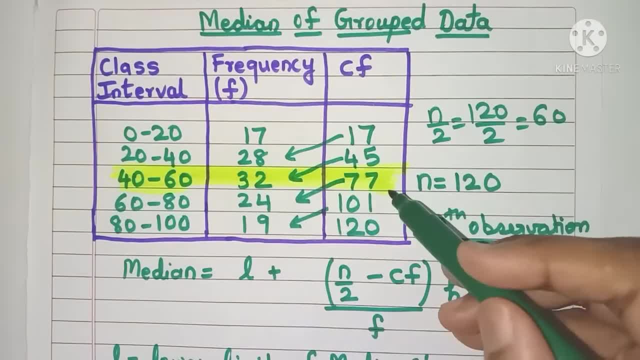 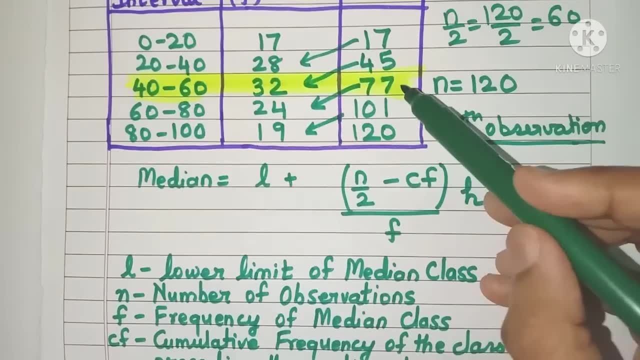 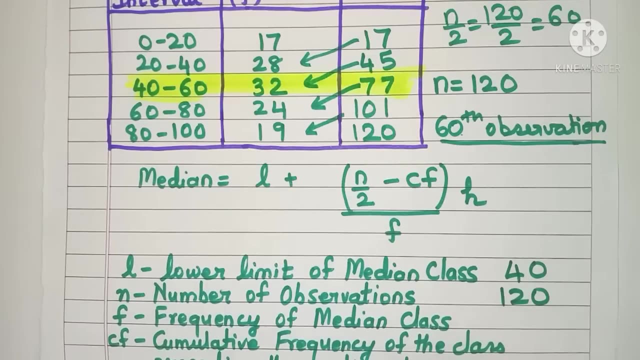 Let's highlight it Now. once we know which is the median class, it's very easy to find the other values also. So, lower limit of median class is L. So which is the median class? This one, Where is the lower limit? 40. So let's write it down. N number of observations. we already know it's 120. 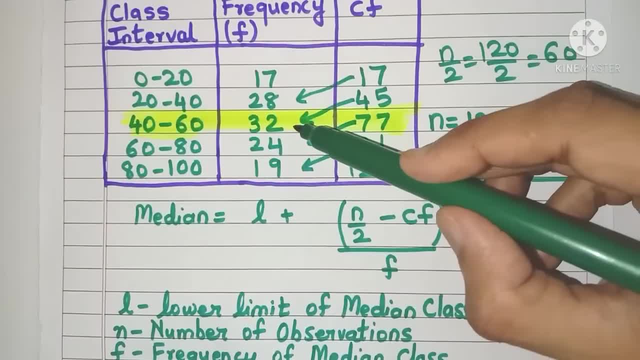 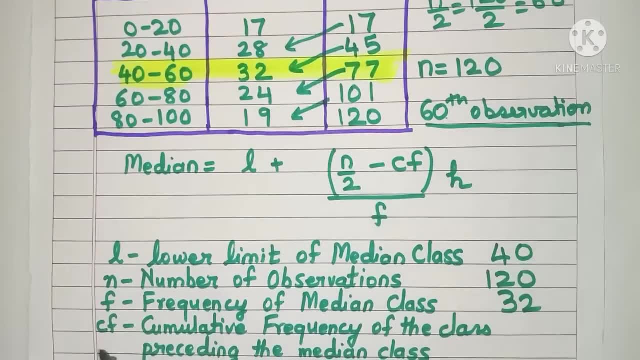 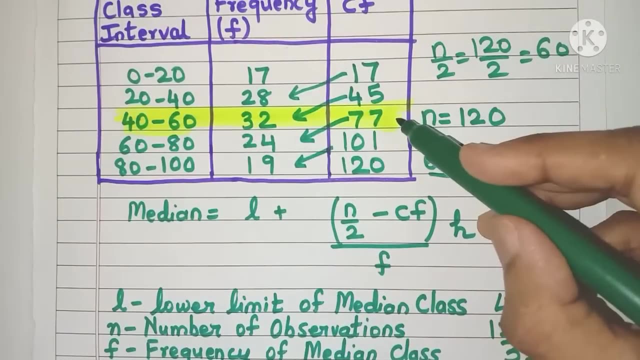 F is frequency of the median class. So what is the frequency of the median class? It's 32.. So let's write it down. Don't confuse F and C, friends, They are totally different. Okay, now the next thing is CF: cumulative frequency of the class preceding the median class. So this is the median 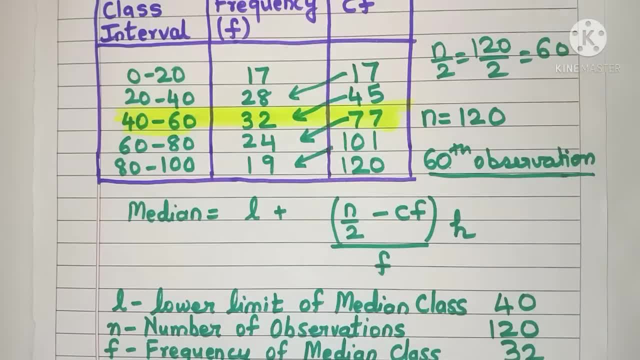 class, the class preceding Preceding means coming before Preceding. the median class is this class? Okay, now what will be the CF of this class? 45. So we have to write here: 45. Friends, don't make. 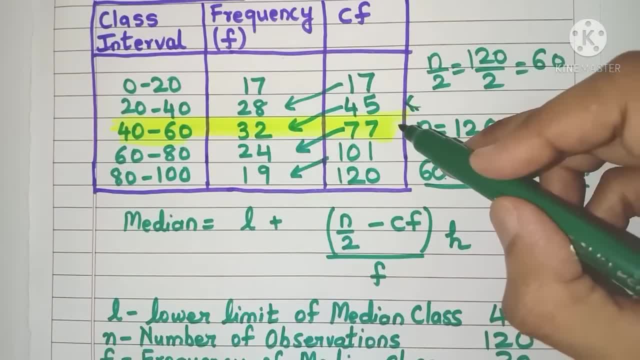 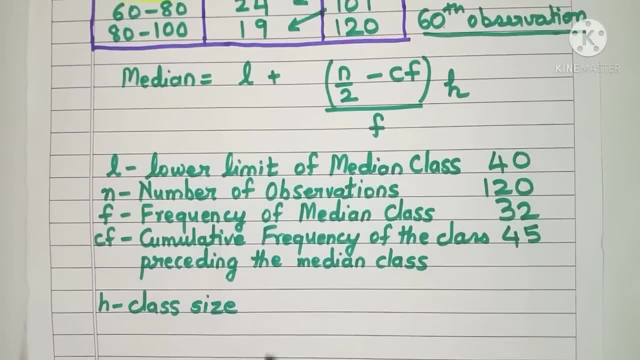 the mistake of writing 77.. Okay, 77 is the CF of the median class. We have to take CF of the class preceding the median class. Okay, Now the next thing we have to find is class size H, which is very easy: 100 minus 80, you take any. 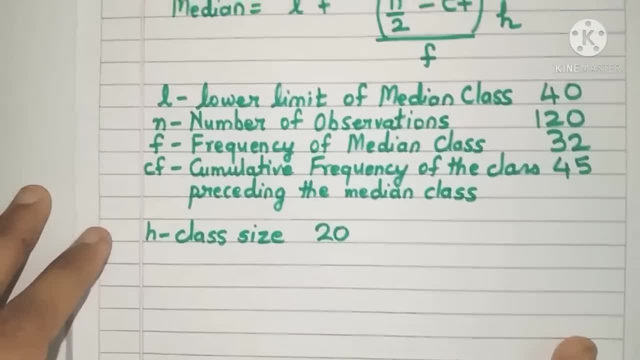 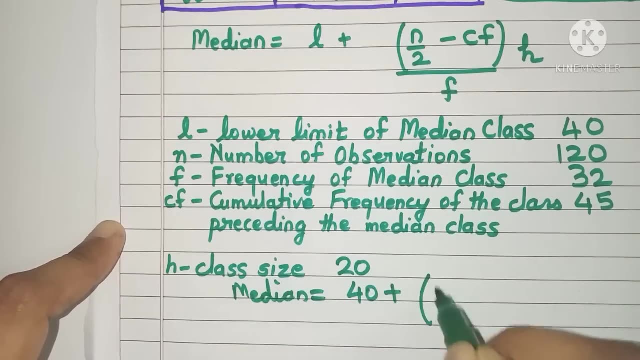 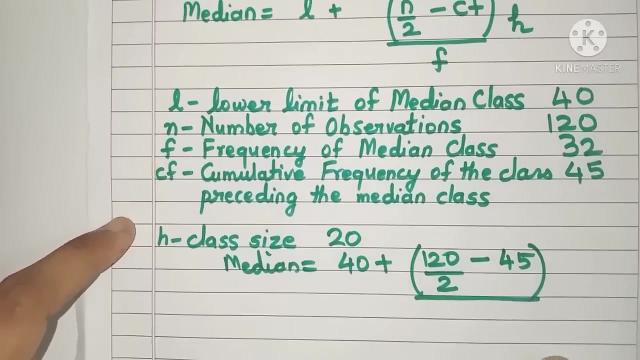 class interval, you'll get it as 20.. Now let's substitute all the values. So median is nothing but L, which is 40 plus N by 2,, 120 by 2 minus CF, which is nothing but 45 divided by the frequency. 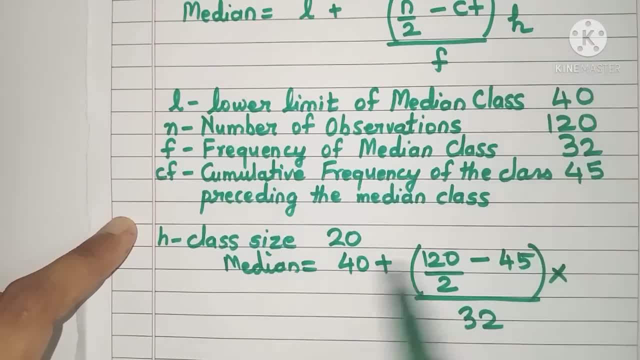 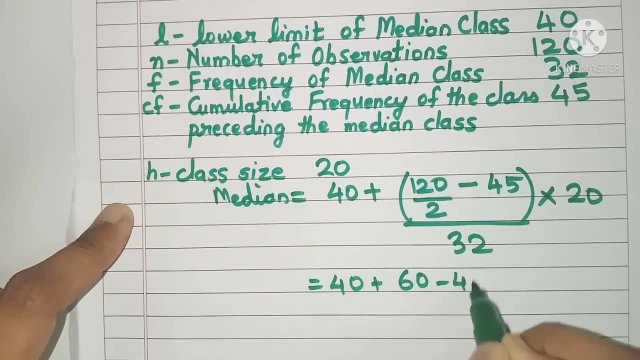 What is it 32 multiplied by H? What is H? Class size: 20.. So let's simplify this further. We'll get 60 minus 45. Keep the bracket 32 into 20.. I think this will go in 4's table no 4. 5's are 20, 4- 8's are 32.. So we will get 40 plus this will become 15.